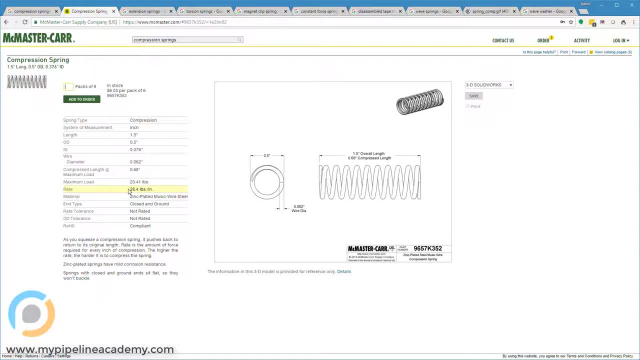 springs. you might be confused, because the rate says 28.4. well, 28.4 is more than 23.4, so what gives? why is that the case? and all that's saying is: this spring is not long enough to be compressed a full inch, and sure enough, we see right here in this row that the the compressed length at the maximum load is 0.68 inches, so we start with 1.5 inches and we get compression down to 0.68 inches, so you get somewhere around 0.8 inches or so of of compression. so that's compression spring. the next one we'll look at is basically the exact opposite of a compression spring. it's a an. extension spring and the. the difference here is that, instead of coils that are spaced out, you're spaced apart like a compression spring that are meant to be pushed together. an extension spring starts with the coils already touching the adjacent coil and there are loops at either end so that you can attach to the spring and pull on it, and so, instead of producing a, a resistive 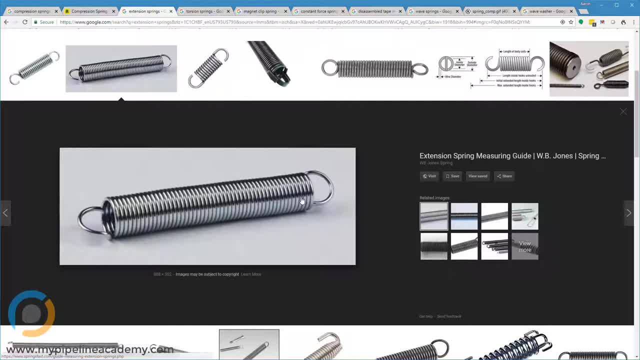 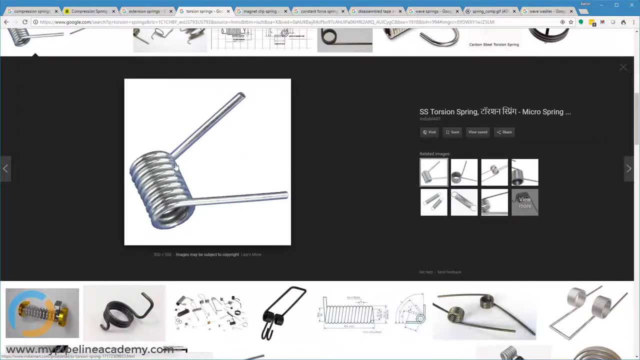 force in compression. this one produces a resistive force in tension. so the first: further you stretch it out you'll get a little bit more force. that you'll see. the next one is torsion Springs, and here's an example of a torsion spring. here these ones produce resistance in a a torsional direction. 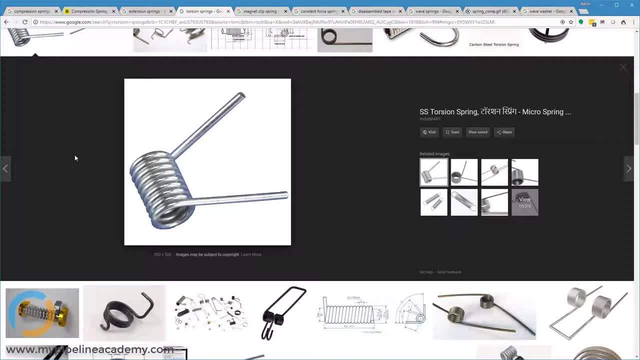 or or a rotational direction, and you often see torsion Springs in things like, you know, hair clips, or they have these, uh, just plastic clips. you know they're used to to like a chip bag. keep a chip bag closed or something like that, or you'll see. 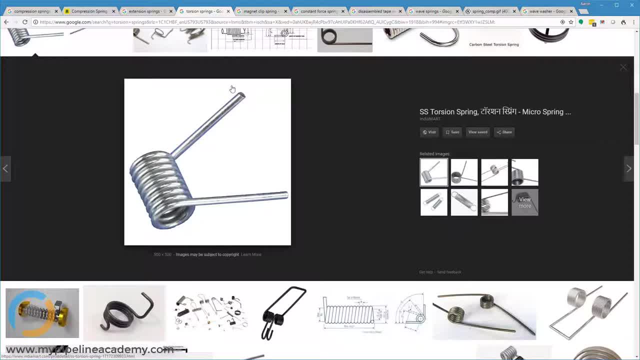 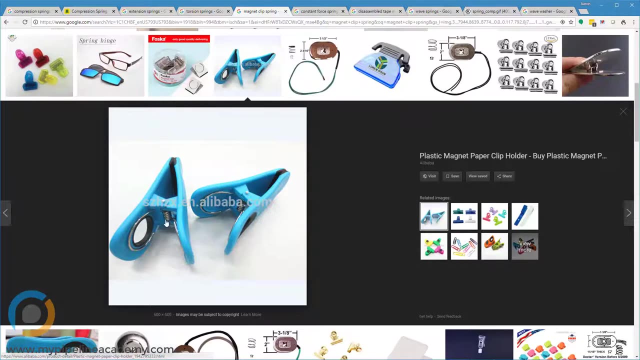 them with magnets on the back and they attach to a refrigerator and it's just a little plastic clip or sometimes a metal clip. those clips are often kept closed by by means of a torsion spring. here's an example. right here you can see this plastic clip and there's the torsion spring in the middle. 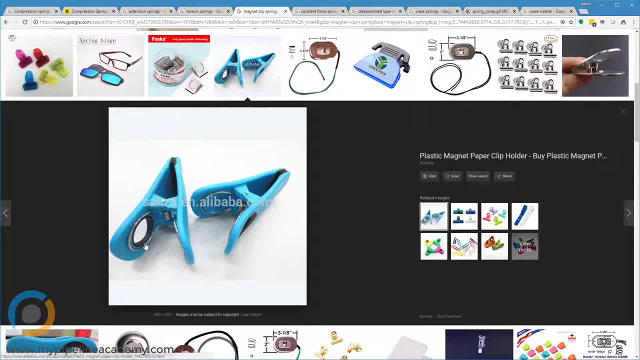 this particular torsion spring has some longer arms, that kind of wrap around like that. um, you can get pretty creative with what your arms look like on a torsion spring. if you're buying off the shelf, then they're usually just going to be straight like this, but if you're making custom, 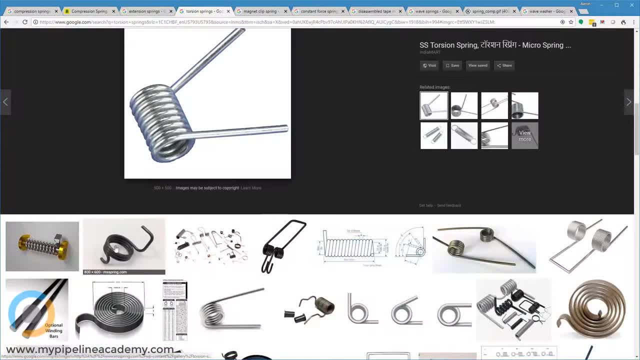 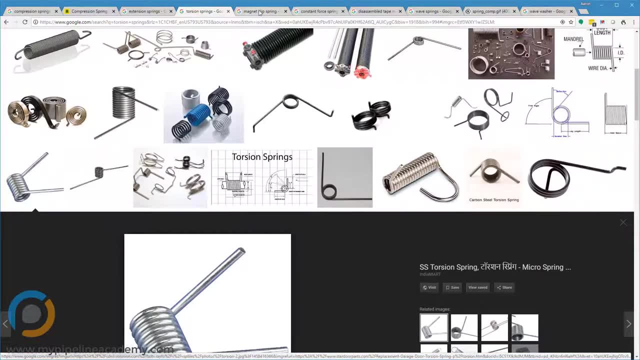 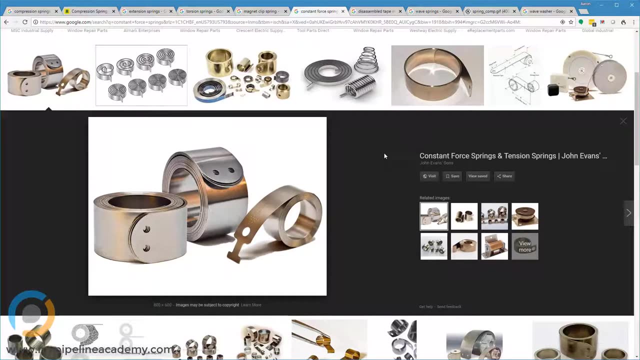 torsion Springs. then you can see down here how there are some pretty creative end Styles on some of these torsion Springs. a few more up here, okay. the next one is a constant force spring, and this is one that that most people never see because it's not typically displayed um in in many real world applications. it's something that's often. 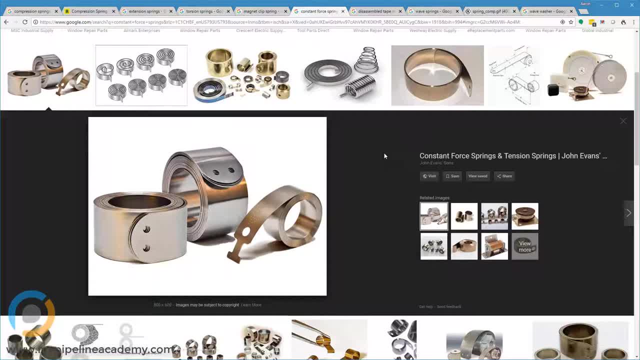 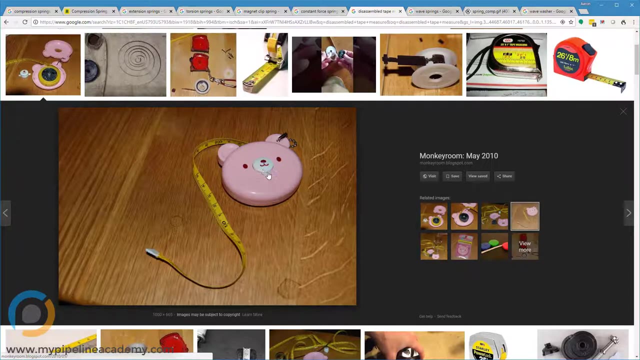 more often than not contained inside some sort of housing and the. a great example of how a constant force spring is used is a tape measure. all tape measures use constant force Springs. that is what provides the um, the, the retraction motion. uh, so if you look at this one here is just kind of a toy tape measure, but it's a functional tape measure. 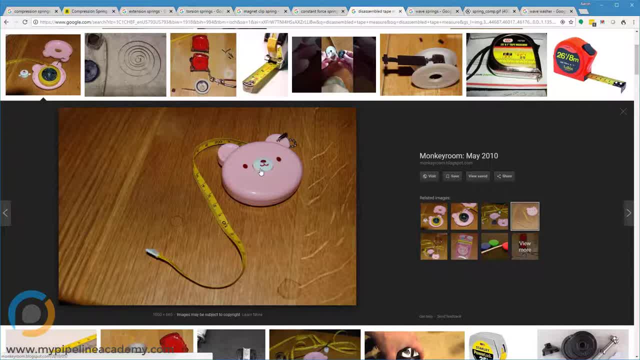 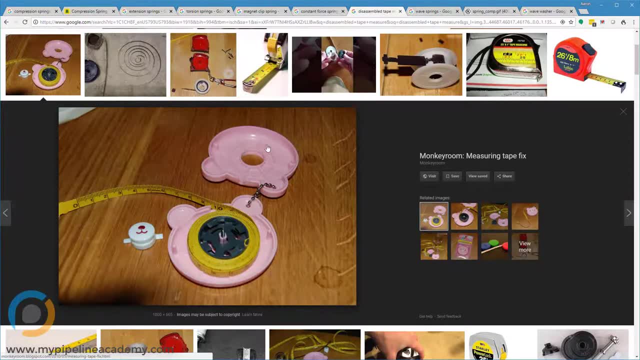 and and the inside of any tape measure is going to look basically the same as this in terms of how it uses a constant force spring. so here are a couple pictures here. it is with the uh one half of the housing removed and you can see the tape measure right there. and then there's this black. 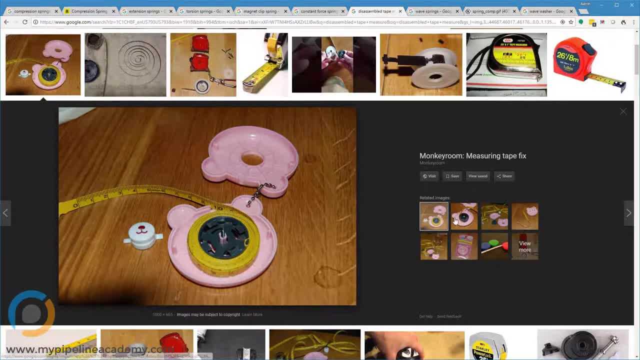 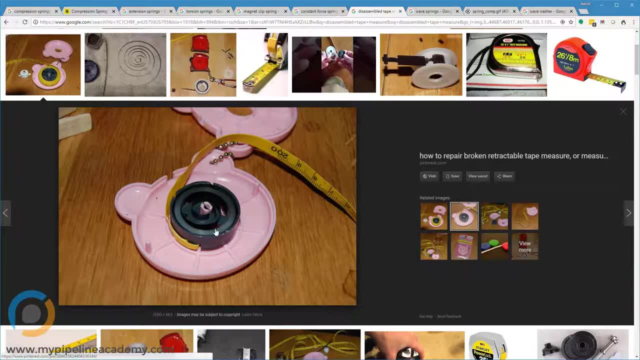 cassette around which the tape is coiled, and then the next picture removes the tape and here you can see there's the, the constant force spring sitting inside that, that cassette right there, and that's what provides that, that rotational motion that pulls your, your tape, in and in and out. constant force Springs, or are great. 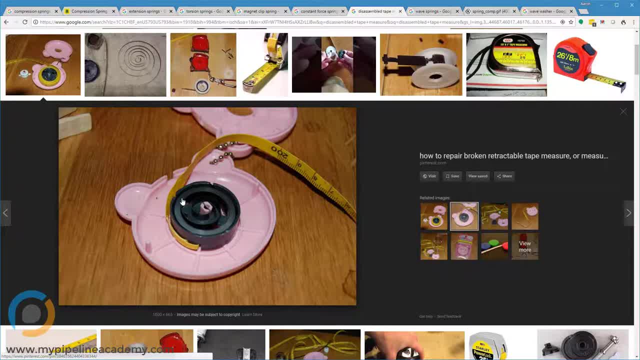 for when you want to have um retracting motion or, you know, tension over a little bit longer length. it could be anywhere from, you know, I don't know, eight, ten inches, up to several feet with the case measure. they're often up to, you know, 30 feet or 40 feet with some of the larger constant force Springs. 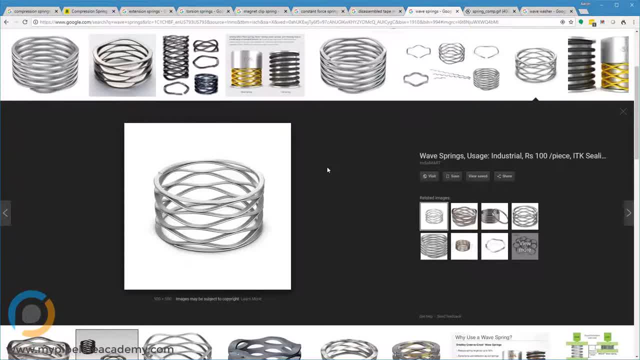 let's see. the next one is a wave spring, and a wave spring is very similar to a compression spring. you can see that they they do differ in their construction, in their architecture, but it performs more or less the same purpose, which is to provide uh, resistance to compression. the difference: is that wave springs will produce more, more force per displacement, so the the spring rate is often a lot higher than than a compression spring, and so what that means is you can get the same amount of force with less, less area, a smaller package size, and that's illustrated in this, this next picture here. 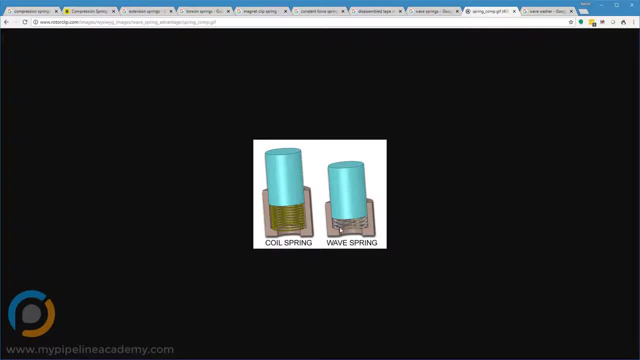 you can see there's a coil spring in one side and a wave spring in the other side. you're getting the same amount of force of resistance but the wave spring. we requires a much smaller space and so a smaller overall package. the trade-off is that wave Springs are more expensive than coil Springs. 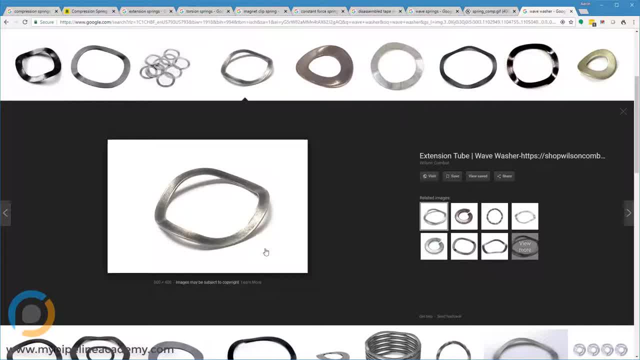 last but not least, we have what's called a wave washer and you can see this wave shape that is formed into. it's just a thin piece of metal, thin washer- and we'll take a look at how that's used in a real world application here next. 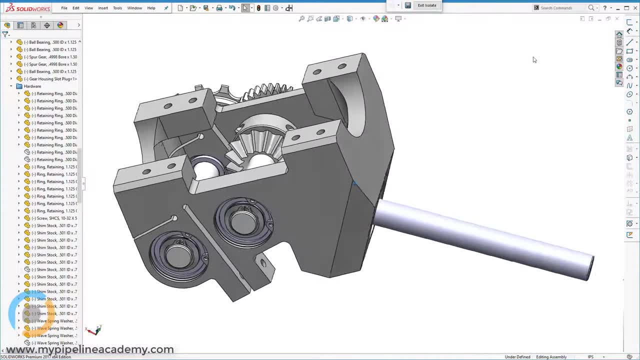 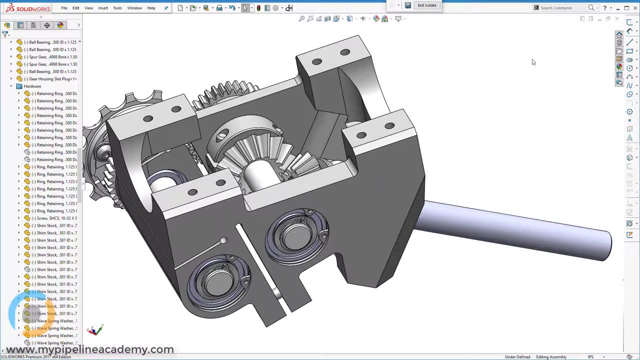 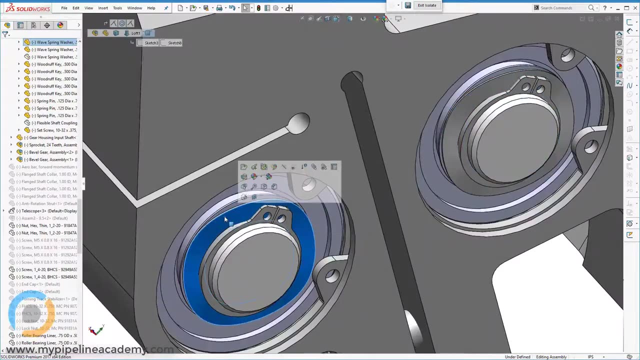 here's a gearbox we looked at in the past and this gearbox actually has some, some wave wave washers, uh, incorporated. so if we zoom in a little bit, here is one of those wave washers and you can see another one here. might have some on the other side, I can't really tell, but uh, these. 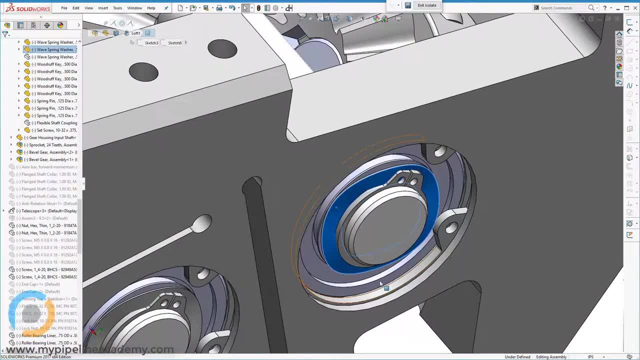 uh, the reason that they're in here is they. they apply just a light axial compression on the inner race of the bearing and, uh, when you're working with bearings in which a shaft, an axle is turning, uh, and you know is turning within a bearing, it's. it's a nice, clean way to. 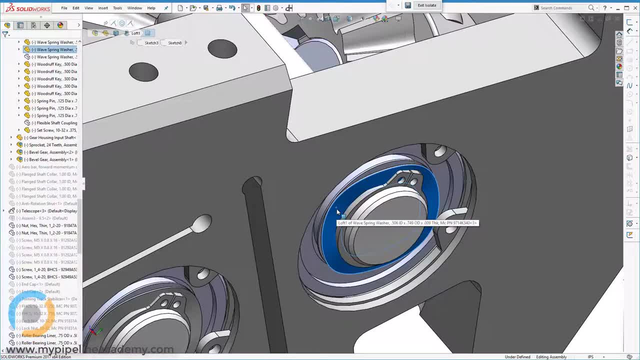 design that interface using a wave washer. they, they just put a little bit of tension on the inner race of that bearing and what happens is, uh, by, by applying a little bit of axial compression on the inner race, it pushes the balls inside the bearing up against the far wall and 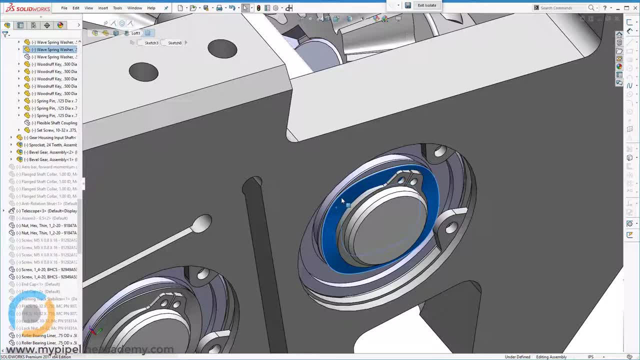 then those balls are, are a nice, you know, light, snug contact with the, the other, the other wall, internal wall of the bearing, and that just allows the bearing to run a little bit smoother, a little bit quieter. so it's a really nice touch when, uh, when, you use one of these little wave or these. 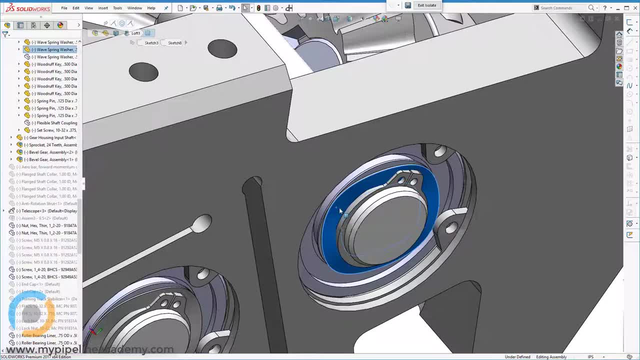 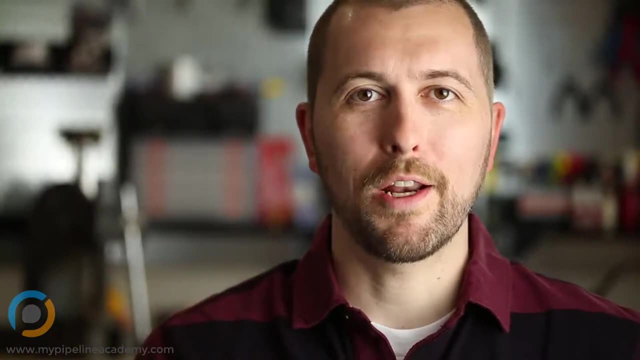 wave washers in your um, in your design um, and so I think that, uh, that covers it, so that'll that'll do it for our lesson on Springs. if you found this content helpful, consider enrolling in our signature program at mypipelineacademycom, whether you're an individual interested in beginning a new. 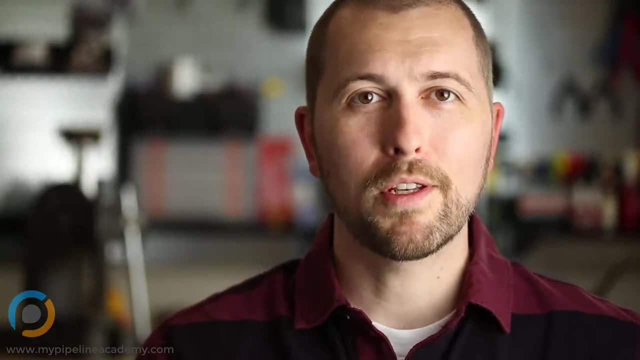 career as a mechanical designer or a company interested in training your new engineering hires. our signature program helps students develop the practical skills they need to be productive mechanical design engineers. seating is limited. we hope to see you there soon.